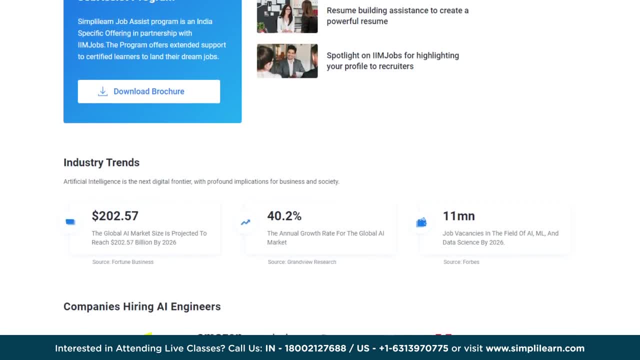 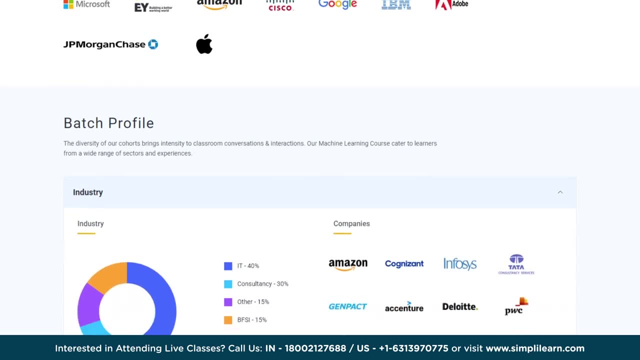 from top universities. After completing these courses, thousands of learners have transitioned into an AI or ML role as a fresher or moved on to a higher-paying job, role and profile. If you are passionate about making your career in this field, then make sure to check out the 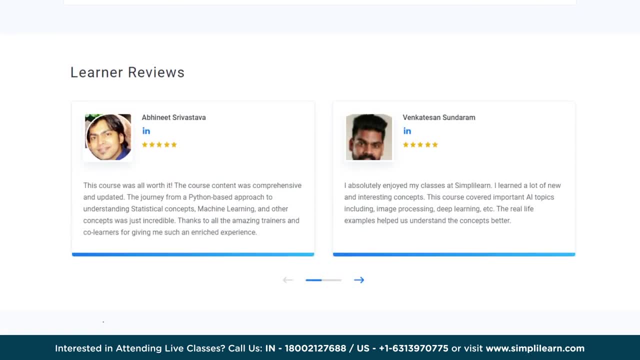 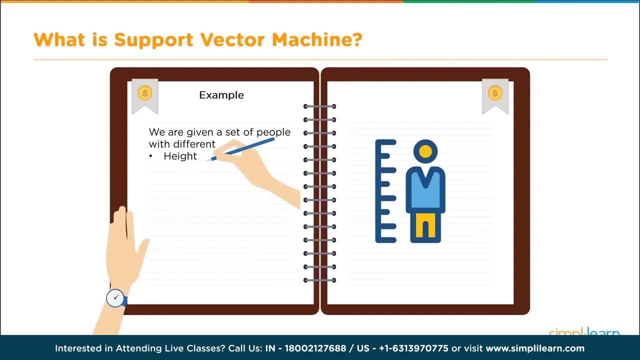 link in the pinned comment and description box to find an AI and ML program that fits your interests. We're going to be classifying men and women And we're going to start with a set of people with a different height and a different weight, And to make this work we'll have to have 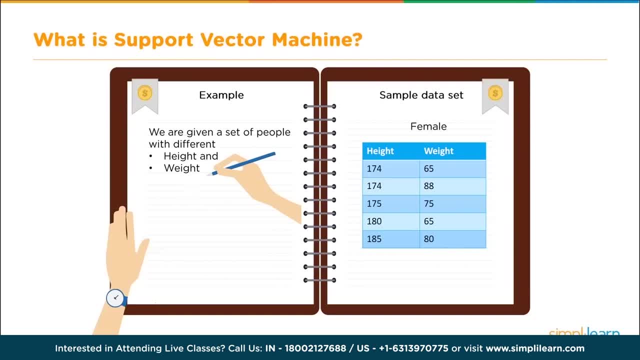 a sample data set of female where you have their height and weight- 174,, 65,, 174,, 88 and so on- And we'll need a sample data set of the male. They have a height 179,, 90,, 180. 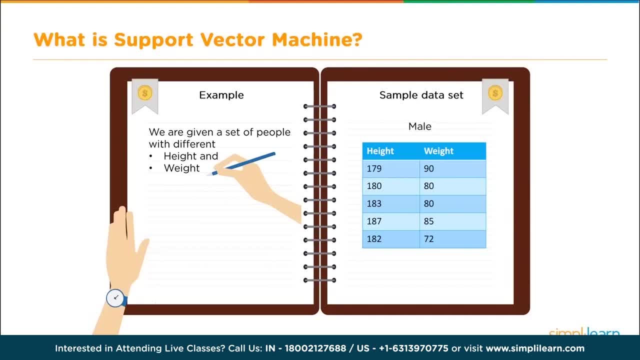 to 80 and so on. Let's go ahead and put this on a graph so you have a nice visual. So you can see, here we have two women And we're going to be classifying men and women And we're going to have two groups, based on the height versus the weight And on the left. 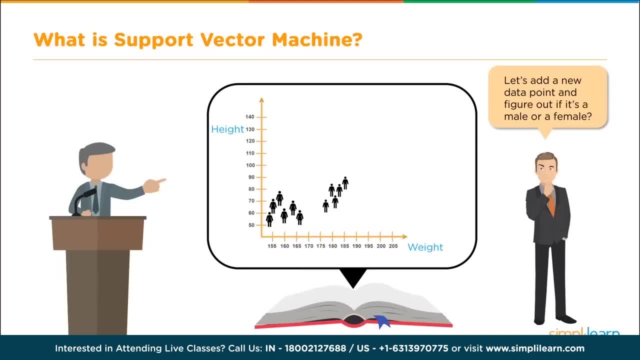 side, we're going to have the women. On the right side, we're going to have the men. Now, if we're going to create a classifier, let's add a new data point and figure out if it's male or female. So before we can do that, we need to split our data first. We can split. 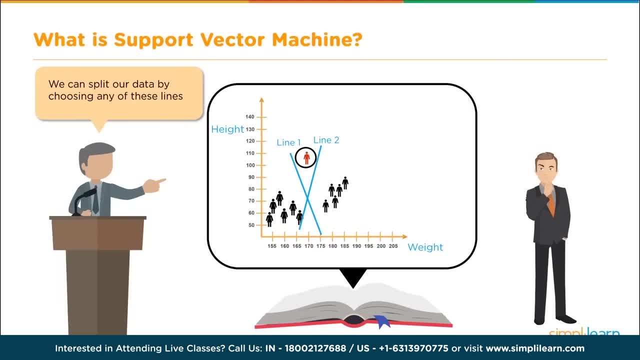 our data by choosing any of these lines. In this case, we've drawn two lines through the data in the middle that separates the men from the women. But to predict the gender of a new data point, we should split the data in the best possible way. 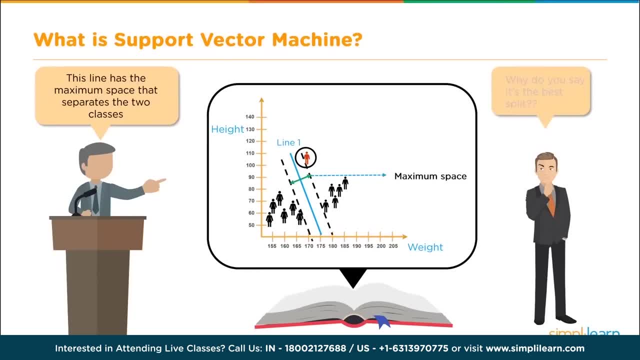 And we say the best possible way, because this line has the maximum space that separates the two classes. Here you can see, there's a clear split between the two different classes And in this one there's not so much a clear split. This doesn't have the maximum space. 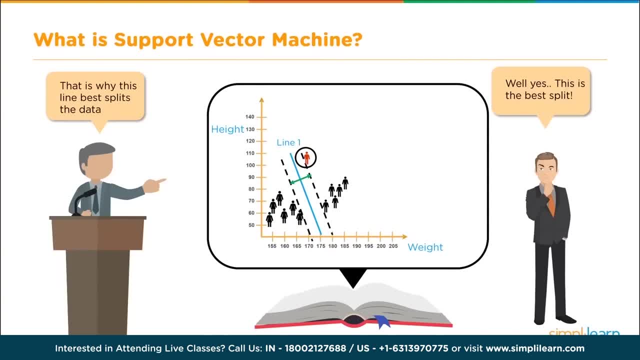 that separates the two. That is why this line best splits the data. We don't want to just do this by eyeballing it, And before we go further, we need to add some technical terms to this. We can also say that the distance between the points and the lines should be: 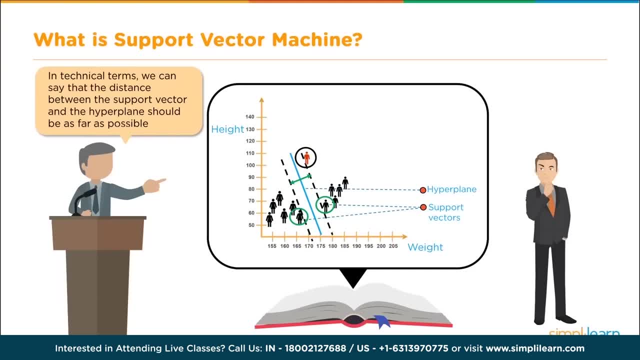 as far as possible. In technical terms, we can say the distance between the support vector and the hyperplane should be as far as possible. And this is where the support vectors are the extreme points in the data set. And if you look at this data set, they 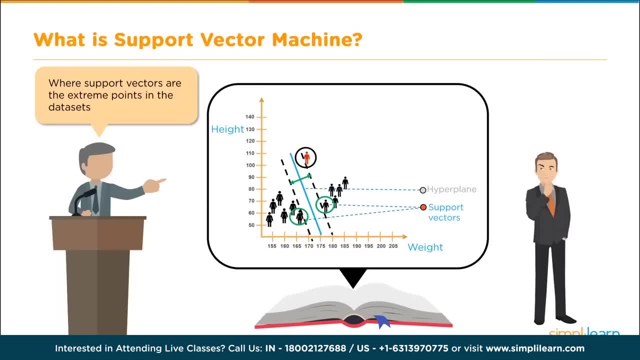 have circled two points which seem to be right on the outskirts of the women and one on the outskirts of the men, And hyperplane has a maximum distance to the support vectors of any class. Now you'll see the line down the middle And we call this the hyperplane. 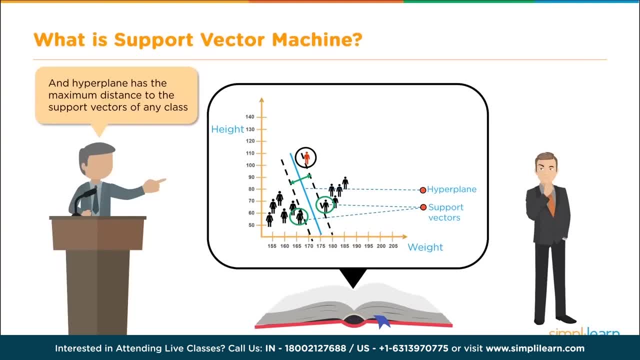 because when you're dealing with multiple dimensions, you're going to have to divide it by the number of lines. It's really not just a line but a plane of intersections, And you can see here where the support vectors have been drawn in dashed lines: The math: 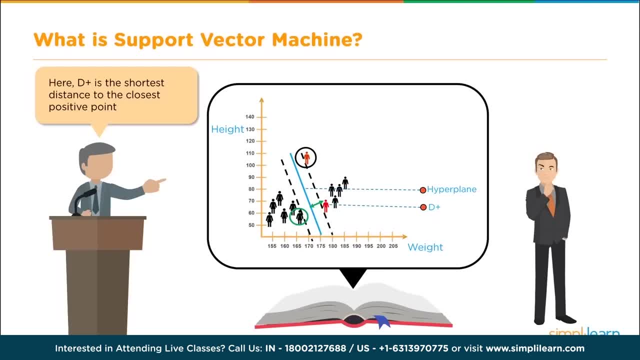 behind. this is very simple. We take D plus, the shortest distance to the closest positive point, which would be on the men's side, and D minus is the shortest distance to the closest negative point, which is on the women's side. The sum of D plus and D minus is called the. 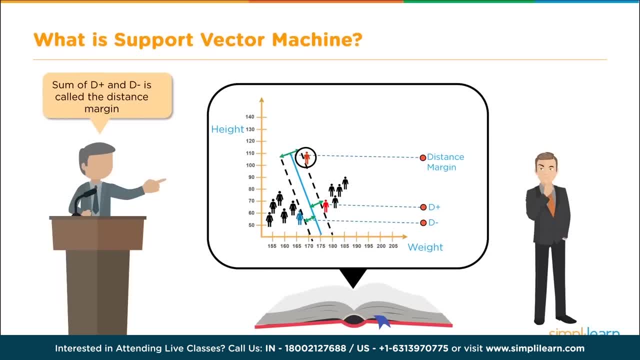 distance margin, or the distance between the two support vectors that are shown in the dashed lines. By finding the largest distance margin, we can get the optimal hyperplane. Once we've created an optimal hyperplane, we can easily see which side the new data fits in And based. 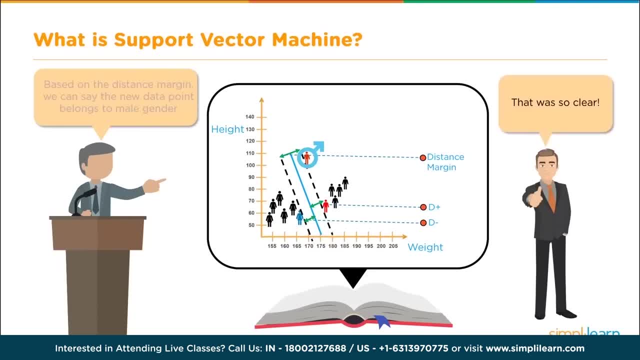 on the hyperplane we can say: the new data point belongs to the male gender. Hopefully that's clear how that works on a visual level. As a data scientist, you should also be asking what happens if the hyperplane is not optimal, If we select a hyperplane having low margin. 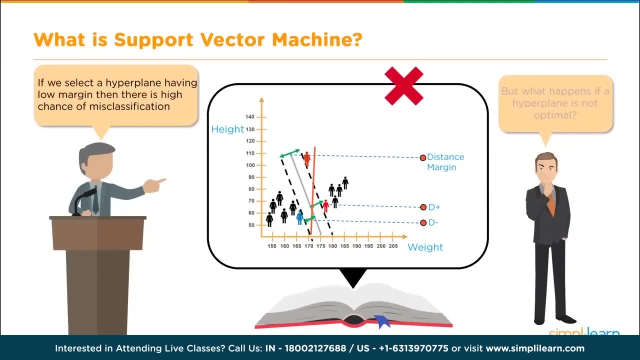 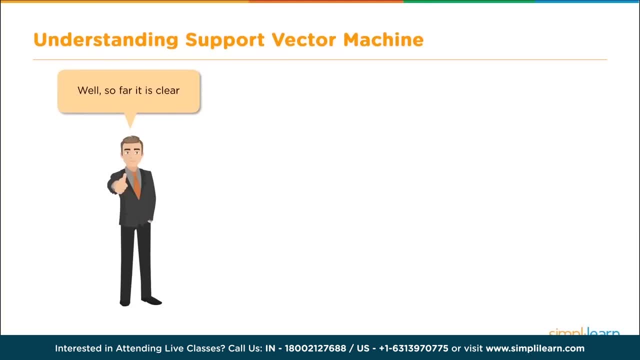 then there is a high chance of misclassification. This particular SVM model, the one we just discussed so far, is also called or referred to as the LSVM. So far, so clear. but a question should be coming up. We have our sample data set, but instead of looking like this, what? 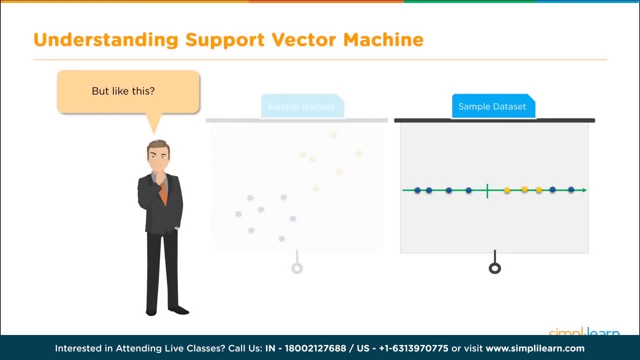 if it looked like this, where we have two sets of data but one of them occurs in the middle of another set. You can see here where we have the blue and the yellow and then blue again on the other side of our data line. In this data set we can't use a hyperplane. 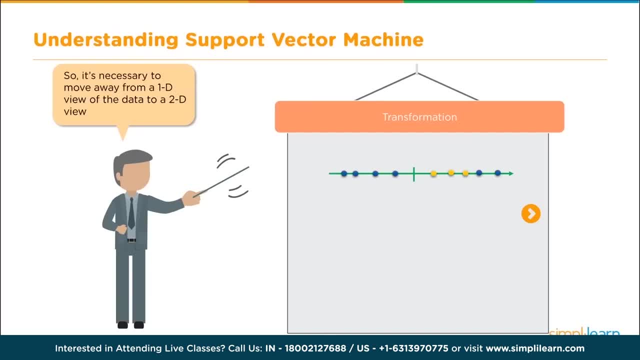 So when you see data like this, it's necessary to move away from the hyperplane and move away from a 1D view of the data to a two-dimensional view of the data, And for the transformation we use what's called a kernel function. The kernel function will take the 1D input and 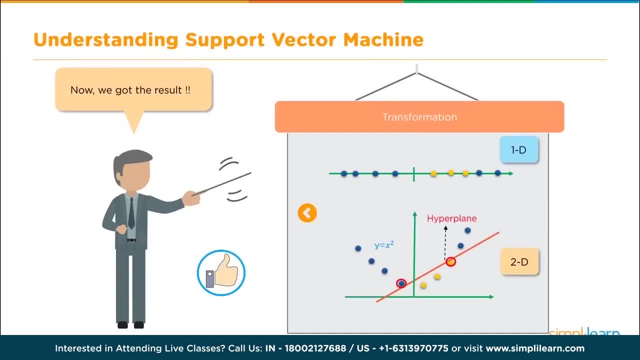 transfer it to a two-dimensional output. As you can see in this picture here, the 1D, when transferred to a two-dimensional, makes it very easy to draw a line between the two data sets. What if we make it even more complicated? How do we perform an SVM for this type of data? 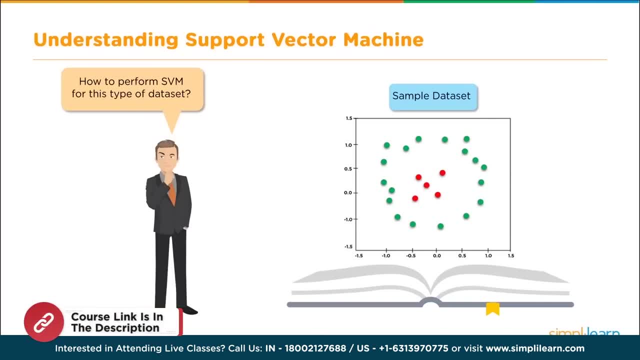 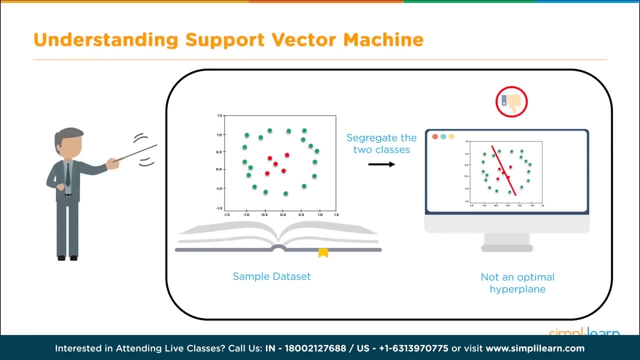 set. Here you can see, we have a two-dimensional data set where the data is in the middle surrounded by the green data on the outside. In this case, we're going to segregate the two classes. We have our sample data set and if you draw a line through, 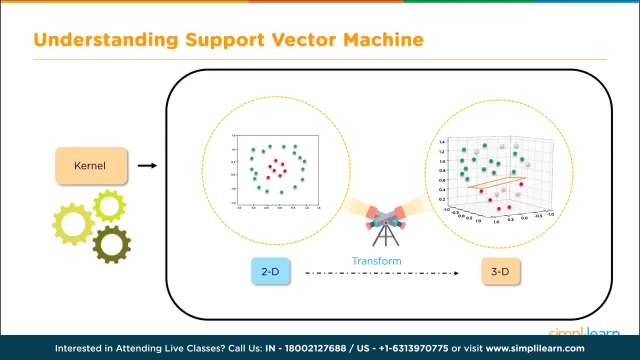 it's obviously not an optimal hyperplane in there. So to do that we need to transfer the 2D to a 3D array, And when you translate it into a three-dimensional array using the kernel, you can see where you can place a hyperplane right through it and easily split. 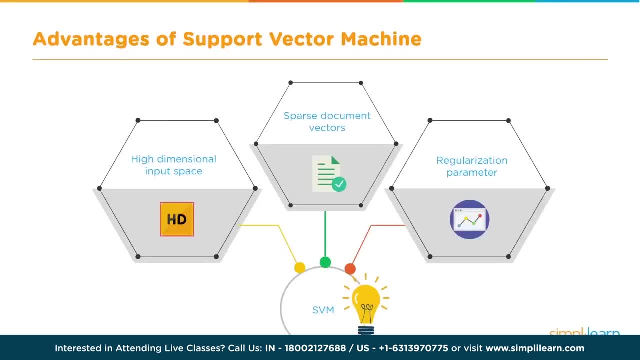 the data. Before we start looking at a programming example and dive into the script, let's look at the advantage of the support vector machine. We'll start with high dimensional input space, or sometimes referred to as the curse of dimensionality. We looked at earlier one dimension, two dimension, three dimension, When you get to a thousand. 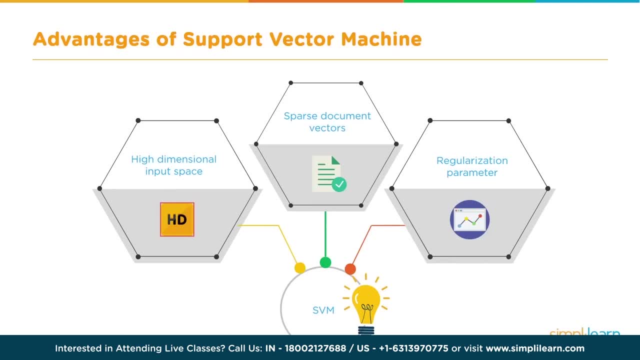 dimensions, a lot of problems start occurring with most algorithms that have to be adjusted for The SVM automatically. does that in high dimensional space? One of the high dimensional space, one high dimensional space that we work on, is sparse document vectors. This is where we tokenize the words and documents so we can run our machine learning algorithm. 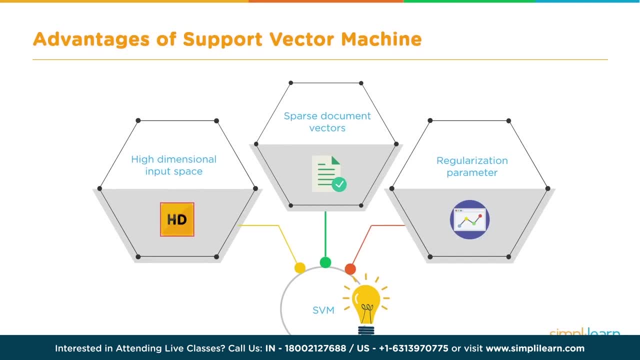 over them. I've seen ones get as high as 2.4 million different tokens. That's a lot of vectors to look at. And finally we have regularization parameter. The regularization parameter, or lambda, is a parameter that helps figure out whether we're going to have 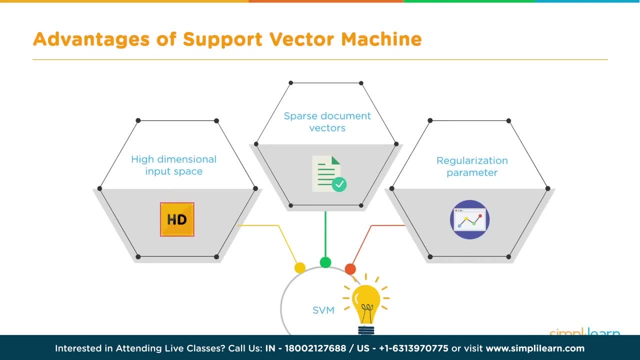 a bias or overfitting of the data, Whether it's going to be overfitted to a very specific instance or it's going to be biased to a high or low value. With the SVM, it naturally avoids the overfitting and bias problems that we see in many other algorithms. These three: 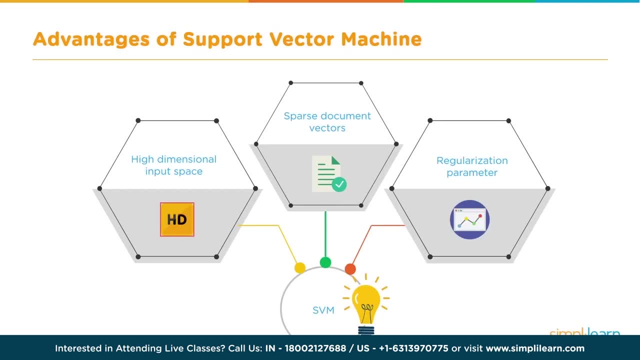 advantages of the support vector machine are the following. The first one is that it's a very powerful tool to add to your repertoire of machine learning tools. Now, we did promise you a use case study. We're actually going to dive into some Python programming, So here. 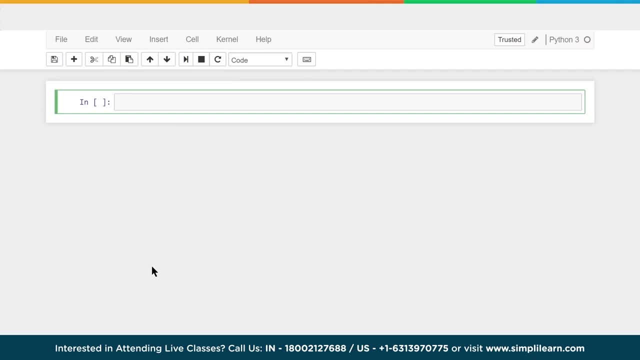 we are in the Anaconda Python notebook or Anaconda Jupyter notebook with Python. We're using Python 3.. I believe this is 3.5, but it should work in any of your 3x versions. You'd have to look at the sklearn to make sure if you're using a 2x version or an earlier. 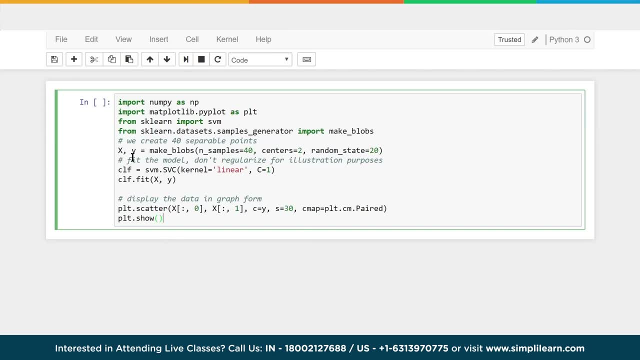 version. Let's go ahead and put our code in there. And one of the things I like about the Jupyter notebook is I can go up to view and I'm going to go ahead and toggle the line numbers on to make it a little bit easier to talk about. 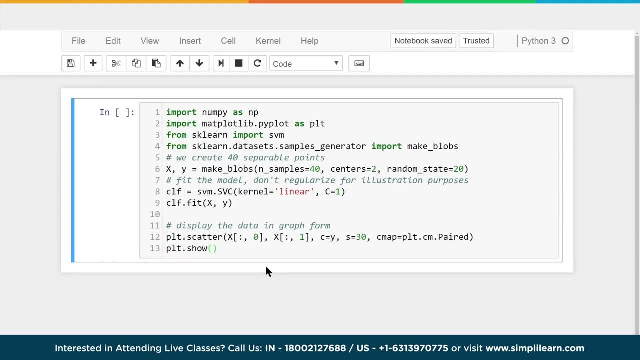 And we can even increase the size, because this is edited in. in this case, I'm using Google Chrome Explorer, and that's how it opens up for the editor, Although anyone, like I said, any editor will work. Now the first step is going to be our imports, And we're going to import four different parts. 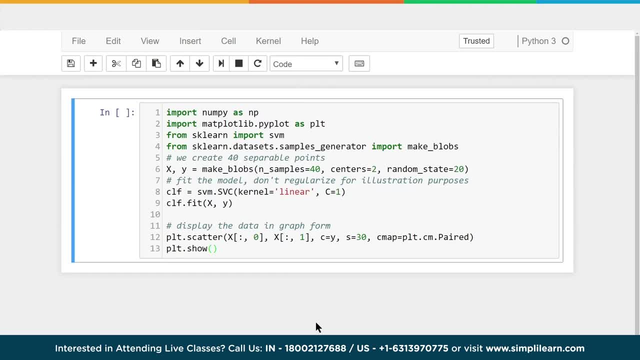 The first two I want you to look at are line one and line two are numpy as np, and matplotlibrarycom. Next to matplot, we also have tuplotlibrarycom, which is the moment we need a start with Now. WE will do this pretty quickly. 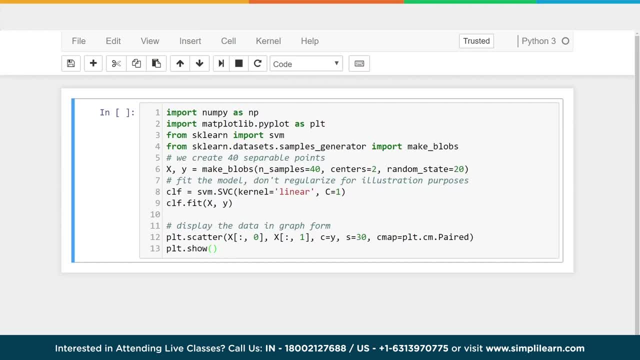 Enansf 1-t sl-ml versus end-esus-1p. We're going to include that now. the map plot library is purely for our use for visualization, and so you really don't need that for the svm. but we're going to put it there so you have a nice visual aid and we can show you. 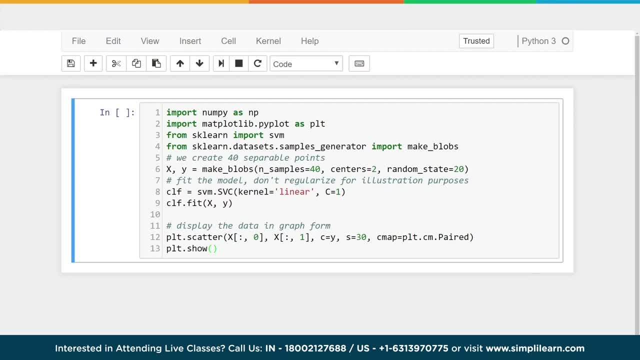 what it looks like. that's really important at the end when you finish everything, so you have a nice display for everybody to look at. and then, finally, we're going to- i'm going to jump one ahead to line number four, that's the sklearndatasetssamples generator. import make blobs, and i told you that. 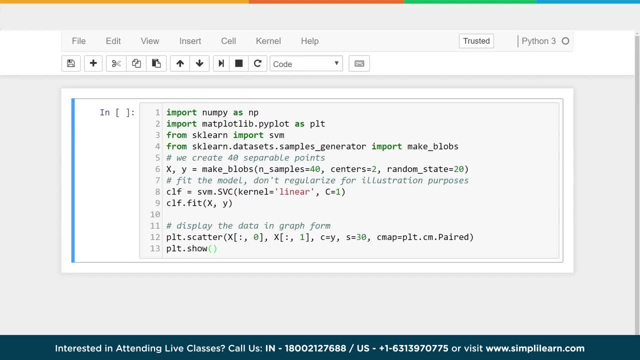 we were going to make up data and this is a tool that's in the sklearn to make up data. i personally don't want to go to the zoo, get in trouble for jumping over the fence and probably get eaten by the crocodiles or alligators as i work on measuring their snouts and width and length. instead, we're 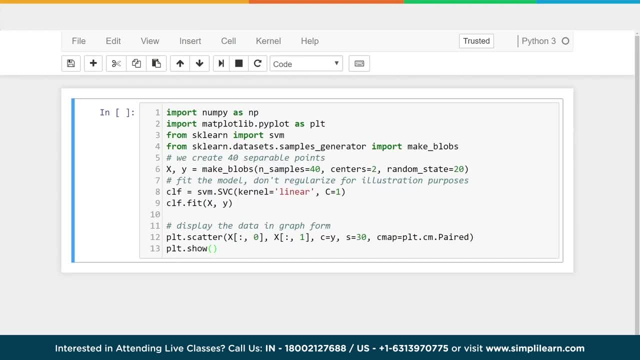 just going to make up some data, and that's what that make blobs is. it's a wonderful tool. if you're ready to test your your setup and you're not sure about what data you're going to put in there, you can create this blob and it makes it real easy to use. and finally we have our actual svm, the sklearn. 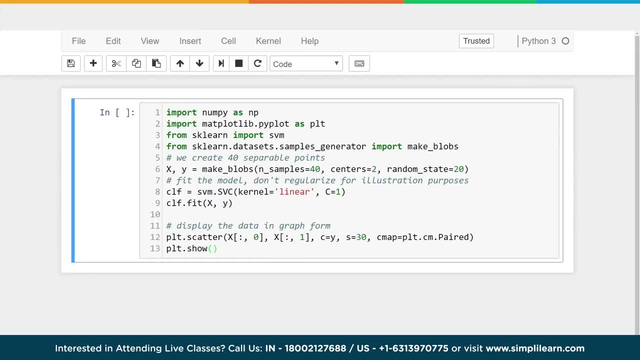 import svm on line three. so that covers all our imports. we're going to create- Remember I used the make blobs to create data- And we're going to create a capital X and a lowercase y equals make blobs in samples equals 40. So we're going to make 40 lines of data. 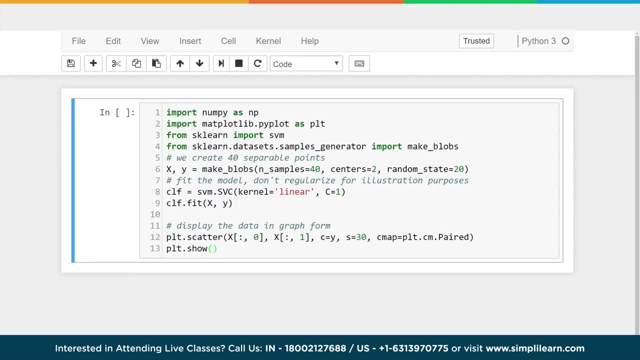 It's going to have two centers with a random state equals 20.. So each group is going to have 20 different pieces of data in it And the way that looks is that we'll have under X an XY plane. So I'll have two numbers under X and Y will be 0 or 1.. 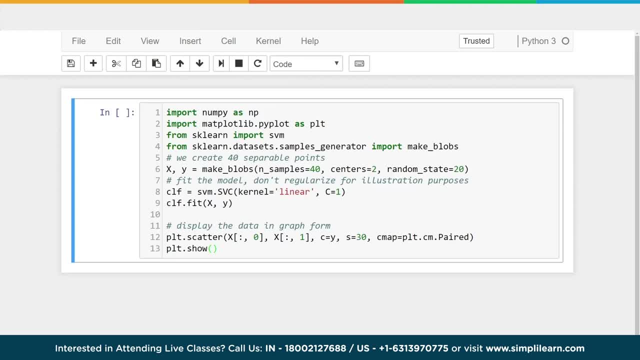 That's the two different centers. So we have, yes or no, in this case alligator or crocodile. That's what that represents. And then I told you that the actual SK learner, the SVM, is in two lines of code And we see it right here with: CLF equals SVM, dot SVC, kernel equals linear. 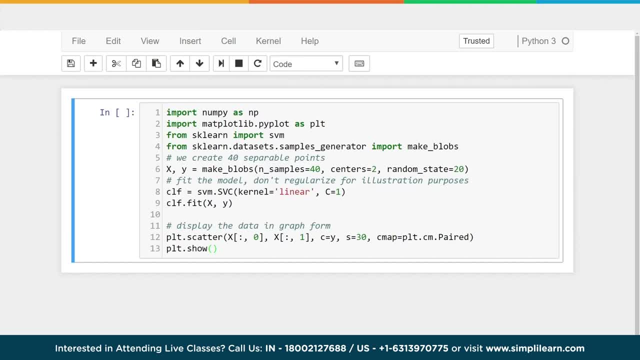 And I set C equal to 1.. Although, in this example, since we are not regularizing the data, since we want it to be very clear and easy to see, I went ahead. you can set it to 1,000 a lot of times when you're not doing that. 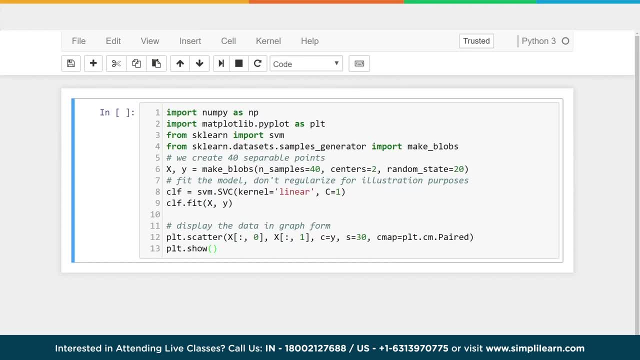 But for this thing, linear because it's a very simple linear. for example, we only have the two dimensions and it'll be a nice linear hyperplane. It'll be a nice linear line instead of a full plane, So we're not dealing with a huge amount of data. 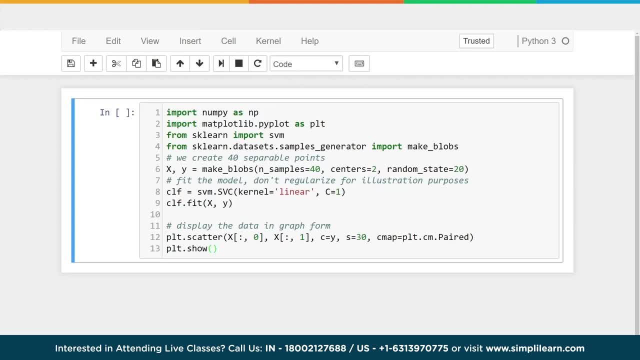 And then all we have to do is do CLF dot fit X, comma Y And that's it. CLF has been created, And then we're going to go ahead and display it, And I'm going to talk about this display here in just a second. 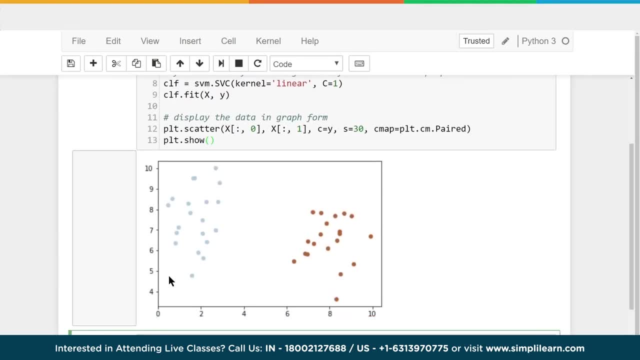 But let me go ahead and run this code, And this is what we've done is we've created two blobs. You'll see the blue on the side and then kind of an orangeish on the other side. That's our two sets of data. 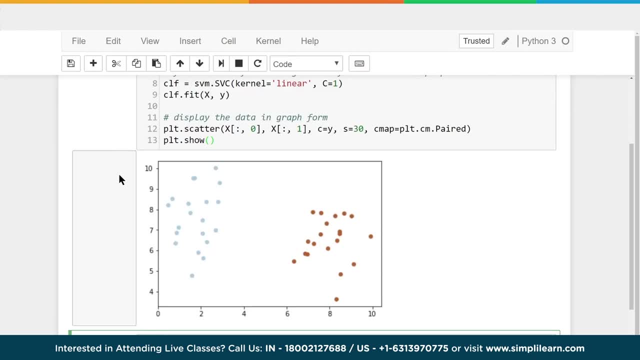 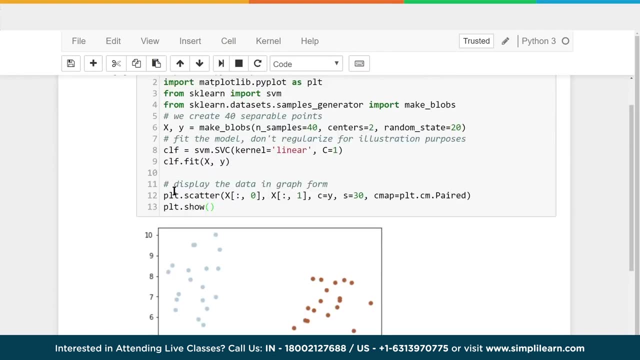 One represents crocodiles and one represents alligators, And then we have our measurements. In this case we have the width and length of the snout, And I did say I was going to come up here and talk just a little bit about our plot. 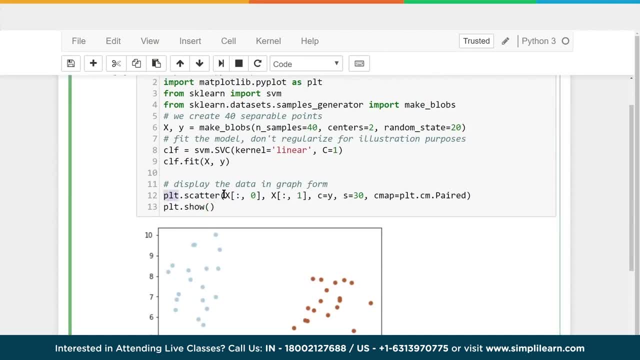 And you'll see PLT. That's what we imported. We're going to do a scatter plot. That means we're just putting dots on there, And then look at this notation: I have the capital X And then in brackets I have a colon, comma 0.. 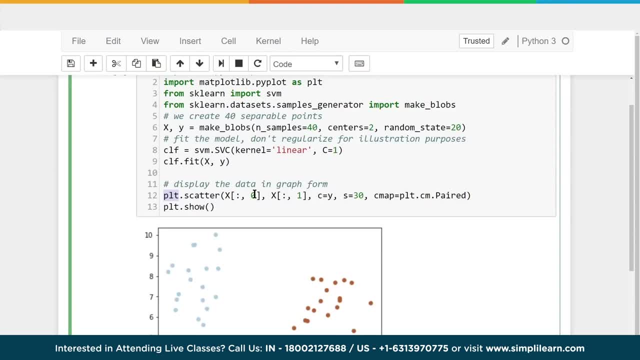 That's from NumPy. If you did that in a regular array, you'll get an error. in a Python array You have to have that in a NumPy array. It turns out that our make blobs returns a NumPy array And this notation is great because what it means 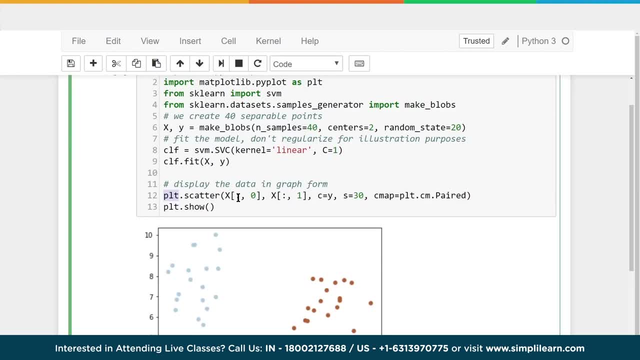 is the first part is the colon. It means we're going to do all the rows. That's all the data in our blob we created under capital X, And then the second part has a comma 0.. We're only going to take the first value. 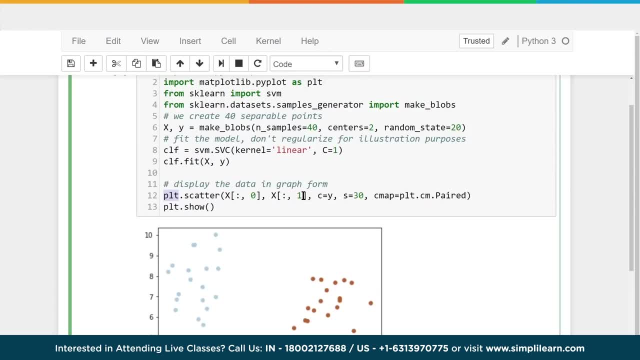 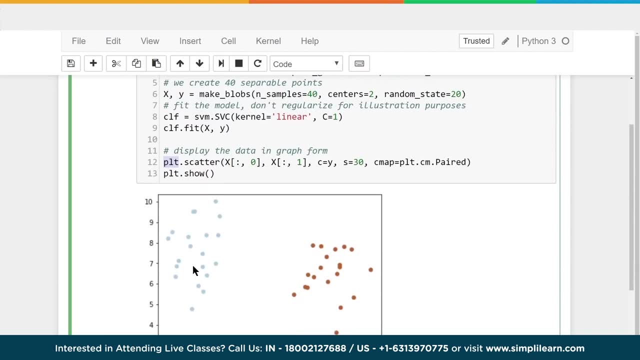 And then, if you notice, we do the same thing, but we're going to take the second value. Remember we always start with 0 and then 1.. So we have column 0 and column 1. And you can look at this as our xy plots. 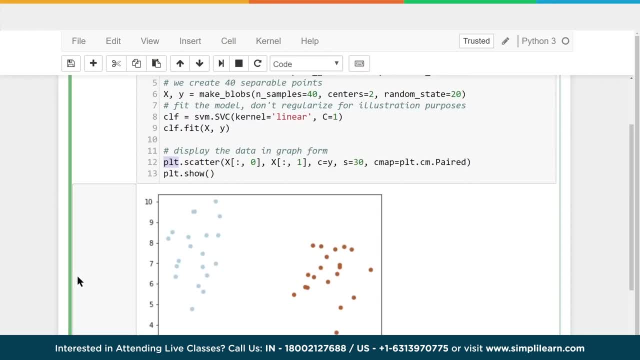 The first one is the x plot and the second one is the y plot. So the first one is on the bottom: 0,, 2,, 4,, 6,, 8, and 10.. And then the second one, x, of the 1,. 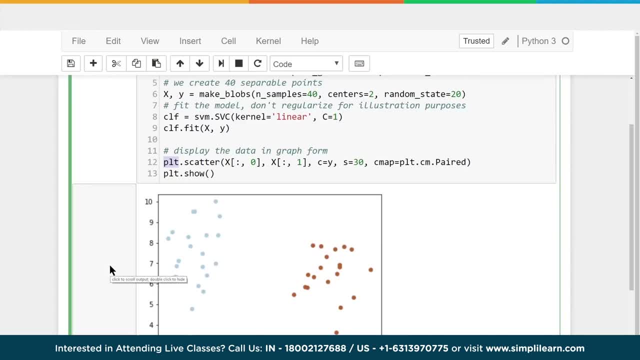 is the 4,, 5,, 6,, 7,, 8,, 9,, 10 going up the left-hand side, S equals 30, is just the size of the dots. We can see them. It's in real tiny dots. 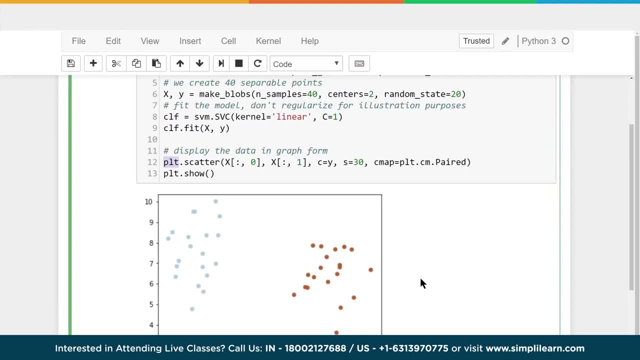 And then cmap equals pltcmpaired, And you'll also see the c equals y. That's the color We're using, two colors: 0, 1.. And that's why we get the nice blue and the two different colors for the alligator and the crocodile. 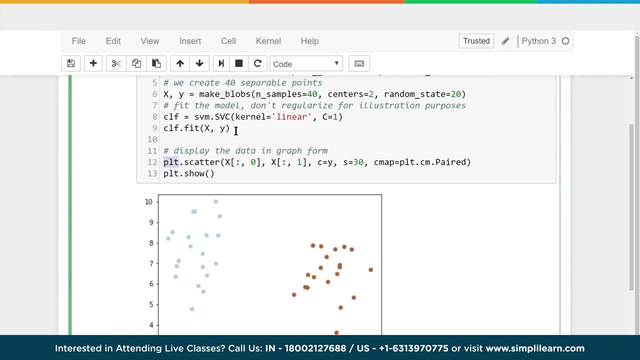 Now you can see here that we did this. The actual fit was done in two lines of code. A lot of times it'll be a third line where we regularize the data, We set it between like minus 1 and 1, and we reshape it. 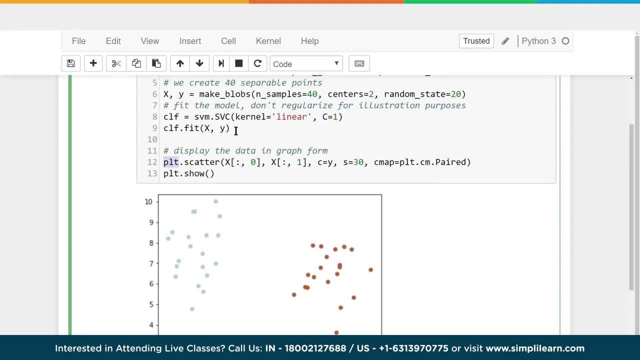 But for this it's not necessary And it's also kind of nice because you can actually see what's going on. And then, if we wanted to, we wanted to actually run a prediction. Let's take a look and see what that looks like. 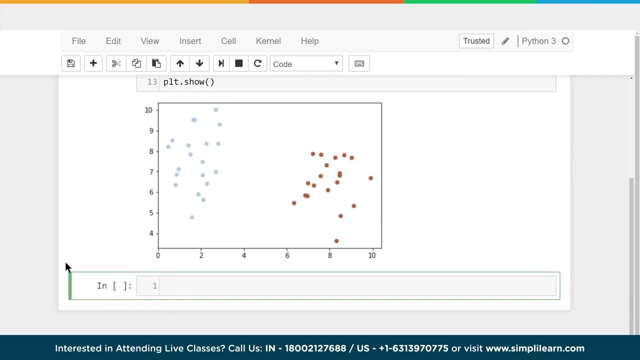 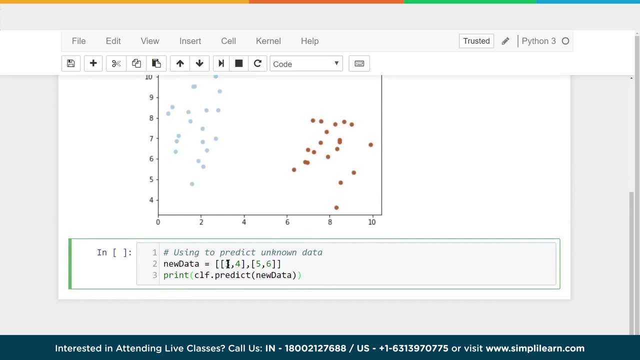 And to predict some new data, and we'll show this again as we get towards the end of digging in deep. you can simply assign your new data. In this case, I am giving it a width and length 3, 4 and a width and length 5, 6.. 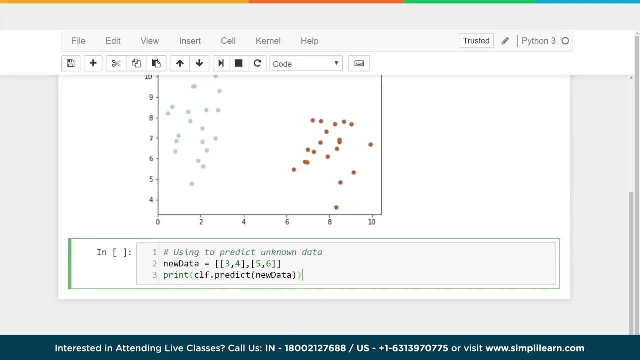 And note that I put the data as a set of brackets And then I have the brackets inside, And the reason I do that is because when we're looking at data, it's designed to process a large amount of data coming in. We don't want to just process one line at a time. 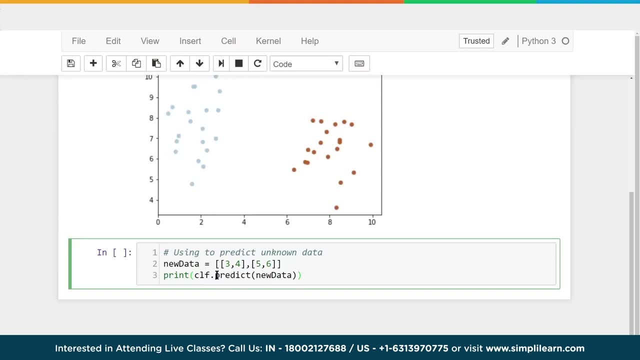 And so in this case I'm processing two lines and then I'm just going to print And you'll see clfpredict new data. So the clf and the predict part is going to give us an answer And let's see what that looks like. 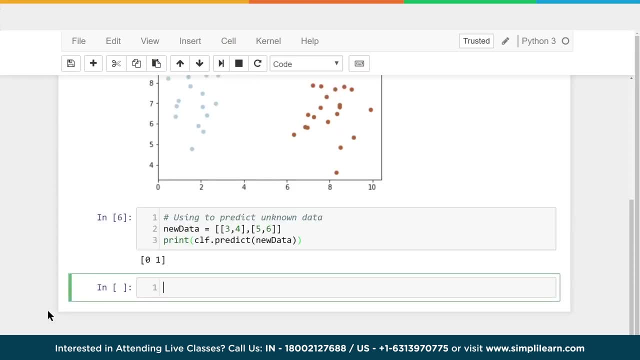 And you'll see 0, 1.. So, predicted, the first one- the 3, 4, is going to be on the one side and the 5, 6 is going to be on the other side. So one came out as an alligator and one 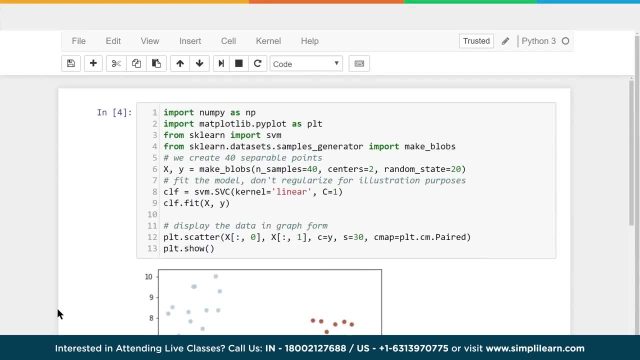 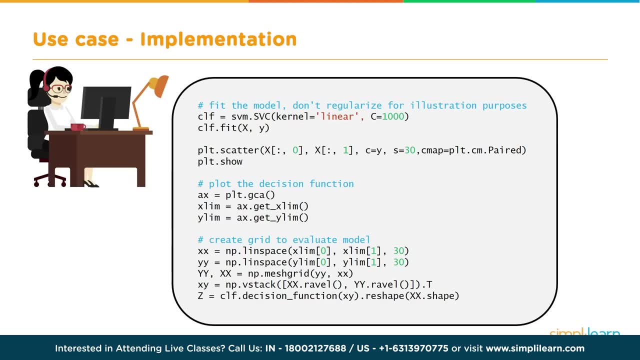 came out as a crocodile. Now, that's a pretty short explanation for this setup, But really we want to dig in and see what is going on behind the scenes And let's see what that looks like. So The next step is to dig in deep and find out. 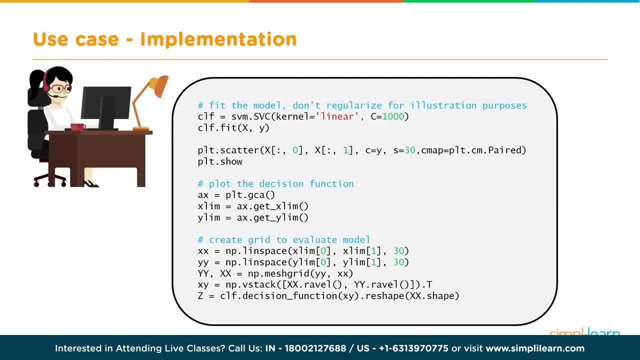 what's going on behind the scenes And also put that in a nice pretty graph. We're going to spend more work on this than we did actually generating the original model, And you'll see here that we go through a few steps And I'll move this over to our editor in just a second. 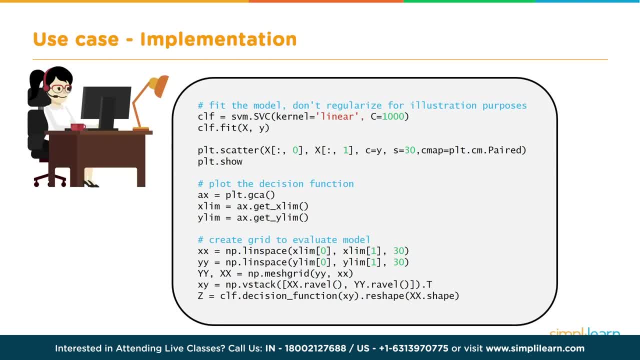 We come in, We create our original data. It's exactly identical to the first part And I'll explain why we redid that and show you how not to redo that. And then we're going to go in there and add in those lines. 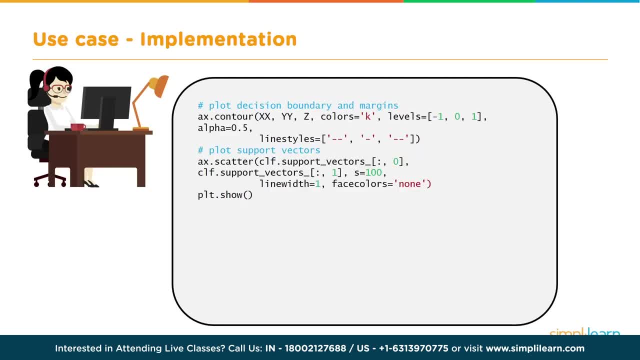 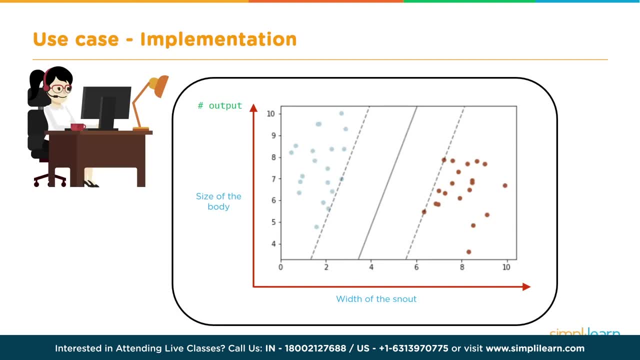 And we're going to see what those lines look like and how to set those up. And finally, we're going to plot all that on here and show it And you'll get a nice graph with what we saw earlier when we were going through the theory. 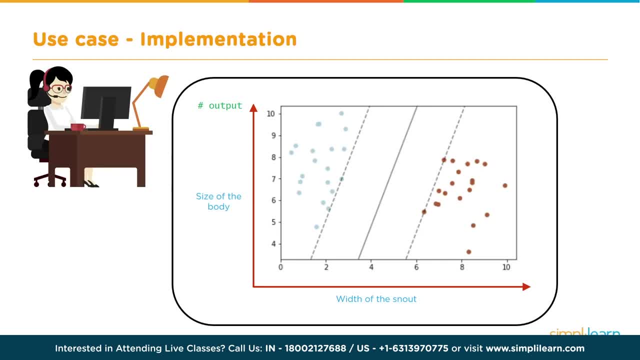 behind this, where it shows the support vectors and the hyperplane And those are done, where you can see the support vectors as the dashed lines and the solid line, which is the hyperplane. Let's get that into our Jupyter notebook Before I scroll down to a new line. 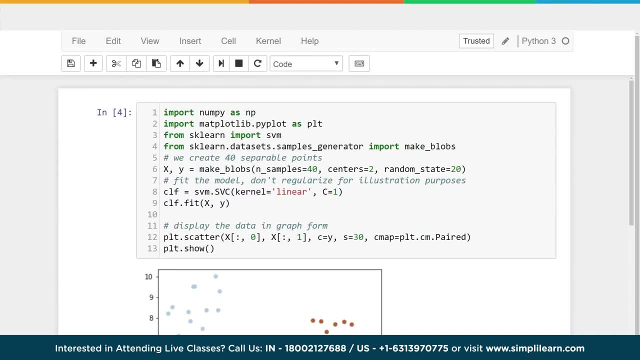 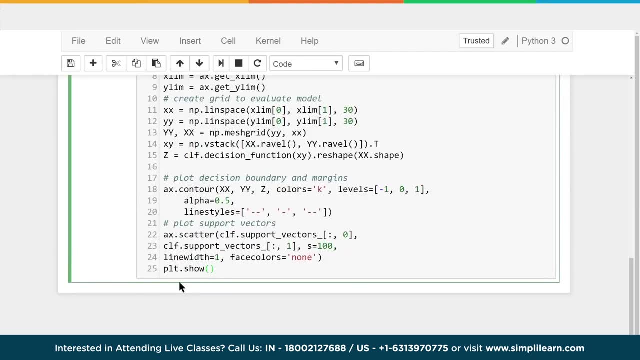 I want you to notice line 13.. It has plot show And we're going to talk about that here in just a second. But let's scroll down to a new line down here And I'm going to paste that code in And you'll see that the plot show has moved down below. 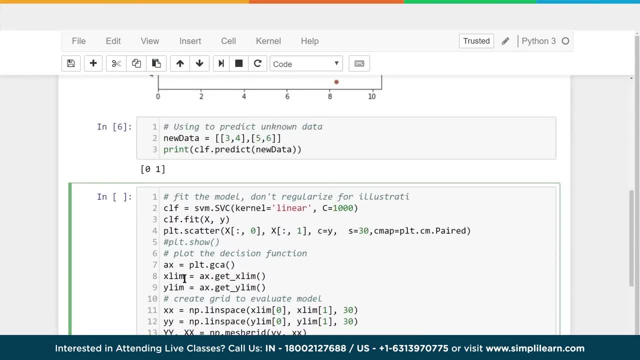 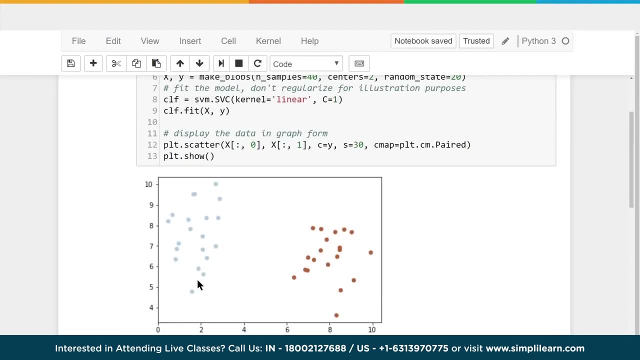 Let's scroll up a little bit And if you look at the top here of our new section, 1,, 2,, 3, and 4 is the same code we had before, And let's go back up here and take a look at that. 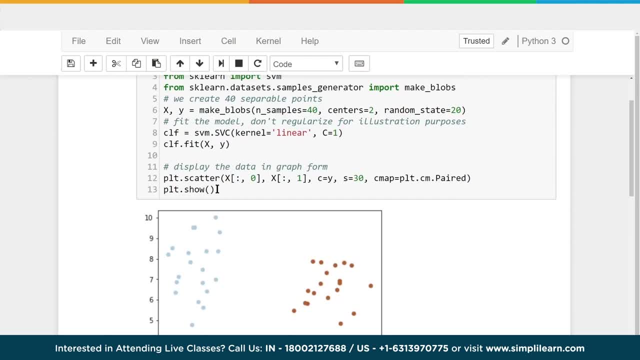 We're going to fit the values on our SVM And then we're going to plot scatter it, And then we're going to do a plot show. So you should be asking: why are we redoing the same code? Well, If you do the plot show, that blanks out what's in the plot. 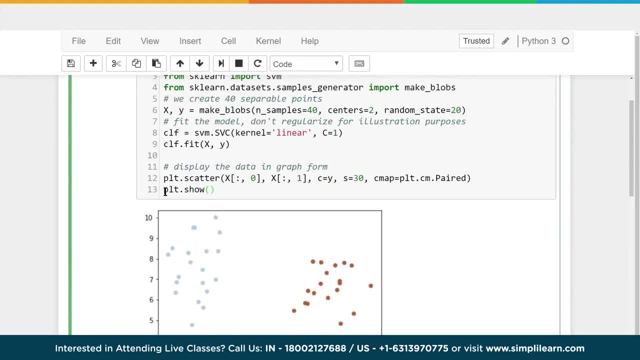 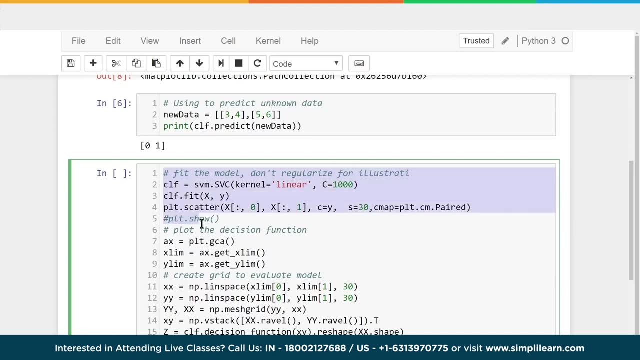 So once I've done this plot show, I have to reload that data. Now we could do this simply by removing it up here, rerunning it and then coming down here, And then we wouldn't have to rerun these first four lines. 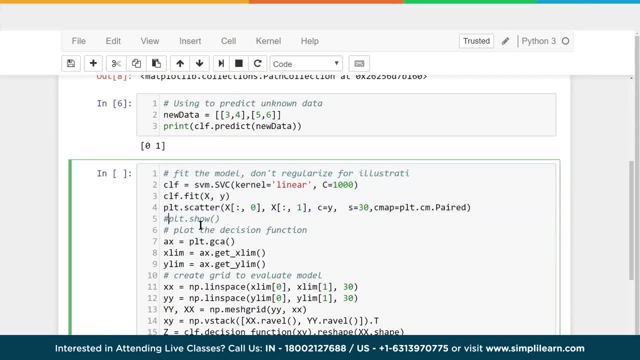 of code Now in this. it doesn't matter too much, And you'll see the plot show is down here and then removed right there on line 5.. I'll go ahead and just delete that out of there, Because we don't want to blank out our screen. 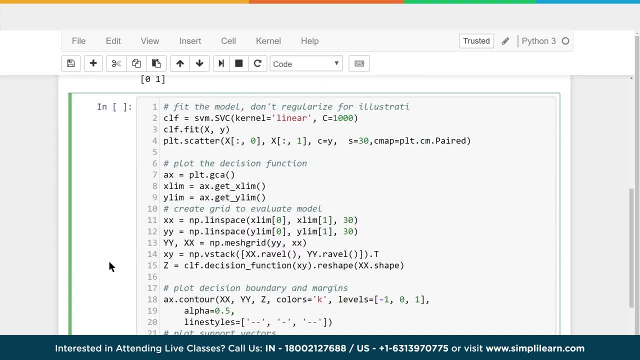 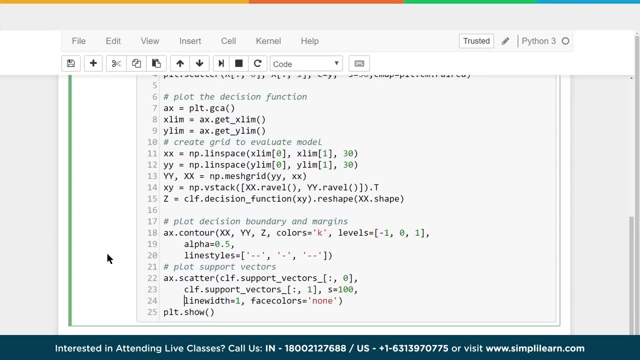 We want to move on to the next setup, So we can go ahead and just skip the first four lines, because we did that before. And let's take a look at the ax equals pltgca Now. right now we're actually spending a lot of time. 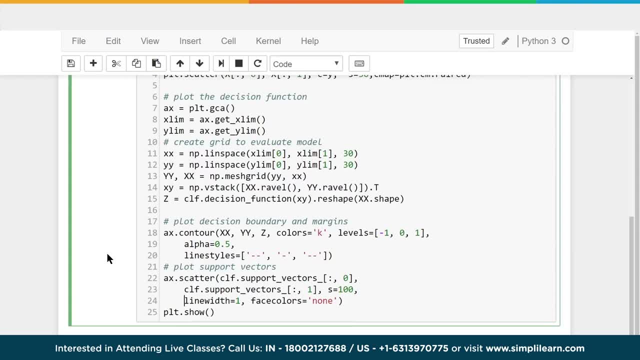 just graphing. That's all we're doing here. So this is how we display a nice graph with our results and our data. Ax is a very standard used variable when you're talking about plt And it's just setting it to that axis, the last axis in the plt. 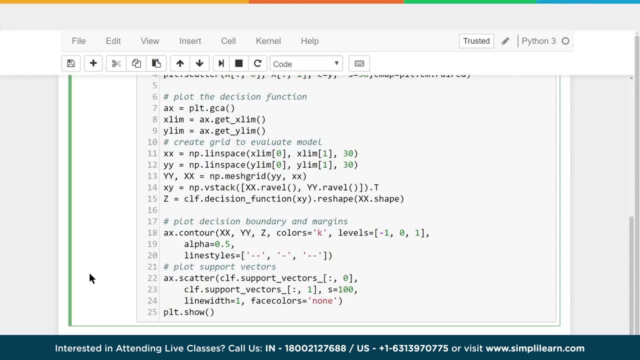 It can get very confusing if you're working with many different layers of data on the same graph, And this makes it very easy To reference the ax. So this reference is looking at the plt that we created, And we already mapped out our two blobs on. 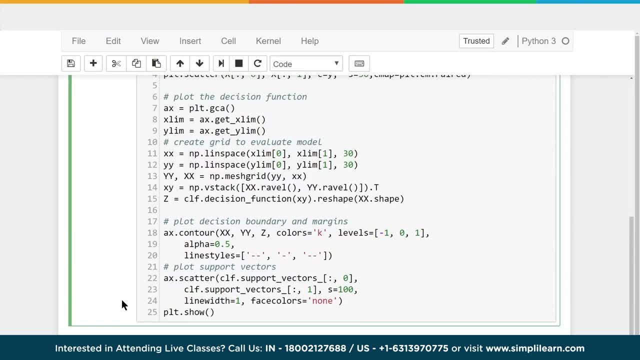 And then we want to know the limits, So we want to know how big the graph is. We can find out the x limit and the y limit simply with the get x limit and get y limit commands, which is part of our matplot library. 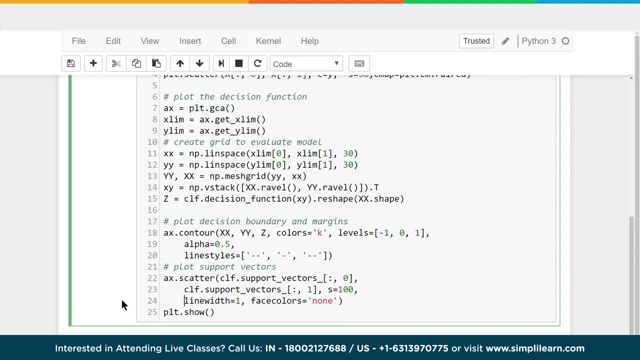 And then we're going to create a grid And you'll see, down here we've set the variable xx, equal to nplinespace, x limit 0,. x limit 1,, 30.. And we've done the same thing for the y space. 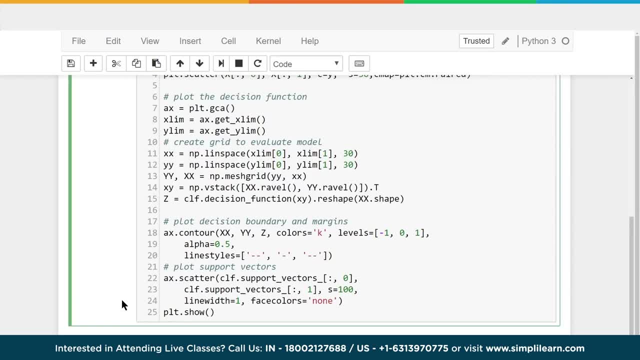 And then we're going to go in here and we create a mesh grid And this is a numpy command. So we're back to our numbers, Python. Let's go through what these numpy commands mean. with the linespace and the mesh grid, We've taken xx small. xx equals nplinespace. 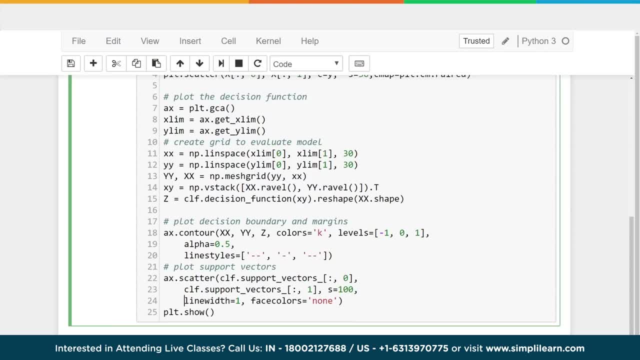 And we have our x limit 0 and our x limit 1.. And we're going to create 30 points on it And we're going to do the same thing for the y axes. Now, this has nothing to do with our evaluation. 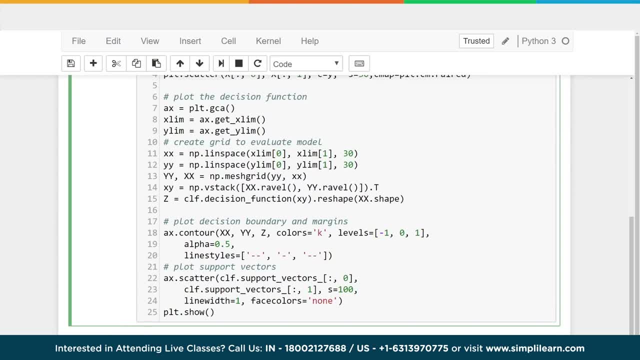 All we're doing is we're creating a grid of data, And so we're creating a set of points between 0 and the x limit. We're creating 30 points And the same thing with the y, And then the mesh grid loops those all together. 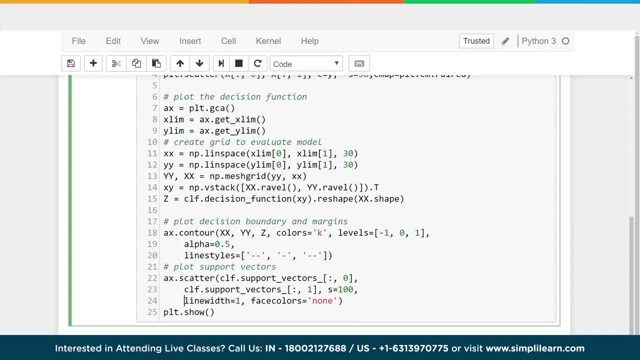 so it forms a nice grid. So if we were going to do this, say between the limit 0 and 10 and do 10 points, we would have a 0, 0, 1, 1, 0, 1, 0, 2,, 0, 3,. 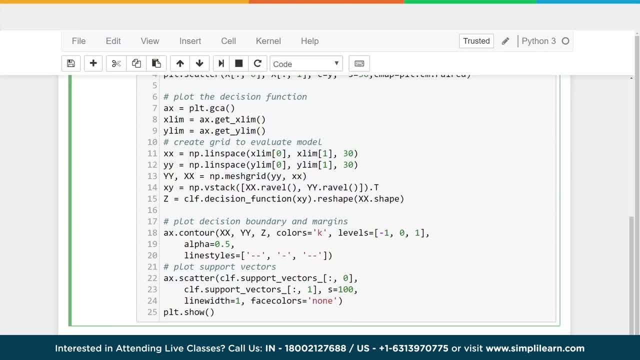 0,, 4, to 10, and so on. You can just imagine a point at each corner of one of those boxes And the mesh grid. It combines them all. So we take the y, y and the x- x we created. 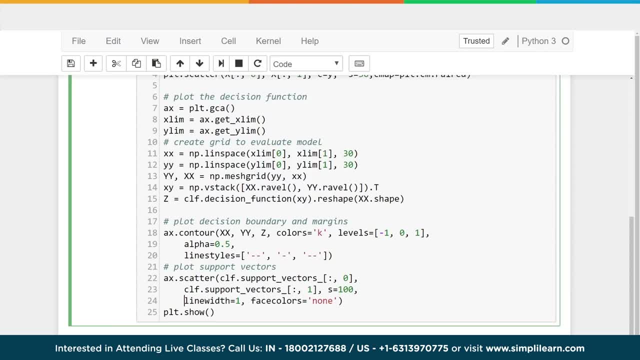 and creates the full grid And we've set that grid into the y- y coordinates and the x- x coordinates. Now, remember we're working with Numbi and Python. We like to separate those. We like to have, instead of it being x 1, x y and then x 2,. 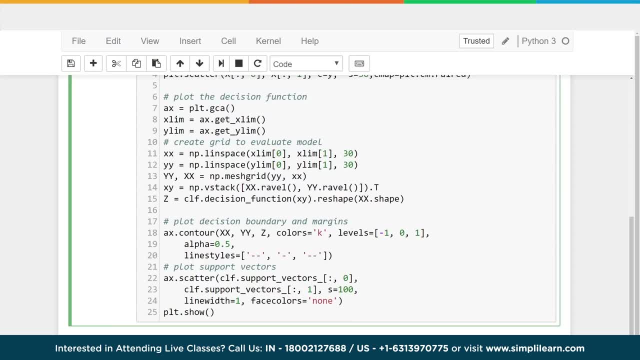 y 2, in the next set of data it would be a column of x's and a column of y's, And that's what we have here is we have a column of y's And we put it as a capital: y, y and a column. 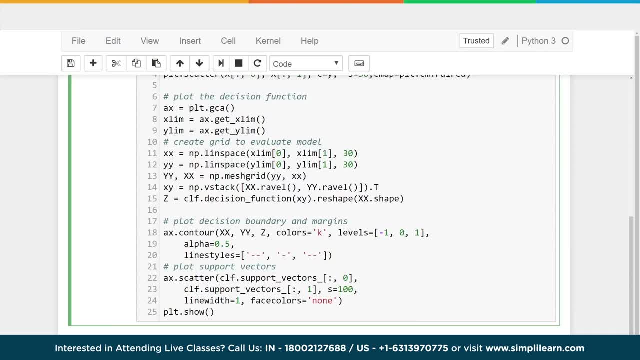 of x's capital, x, x, with all those different points being listed And finally we get down to the Numbi VStack. Just as we created those in the mesh grid, we're now going to put them all into one array: x, y array. 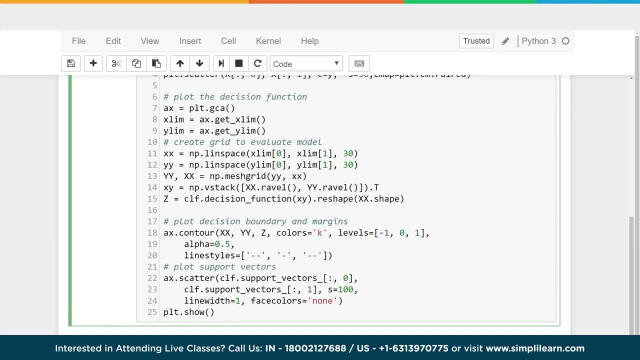 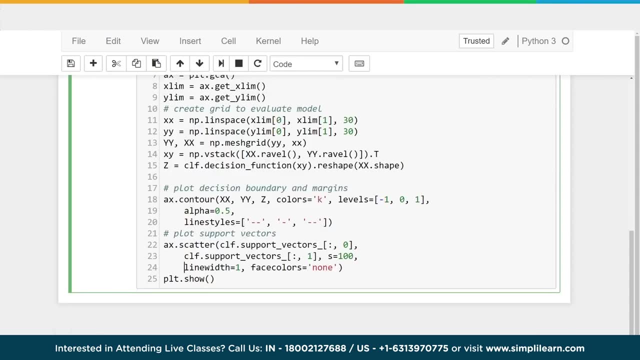 Now that we've created the stack of data points, we're going to do something interesting here. We're going to create a value, z, And the z equals the CLF. That's our support vector machine. we created and we've already trained. 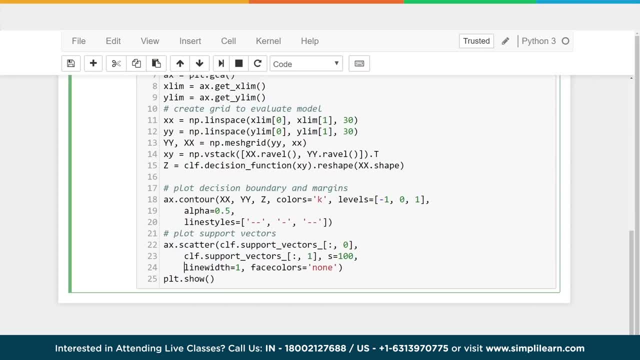 And we have a dot decision function And we're going to put the x- y in there. So here we have all this data, We're going to put that x- y in there, that data, And we're going to reshape it. 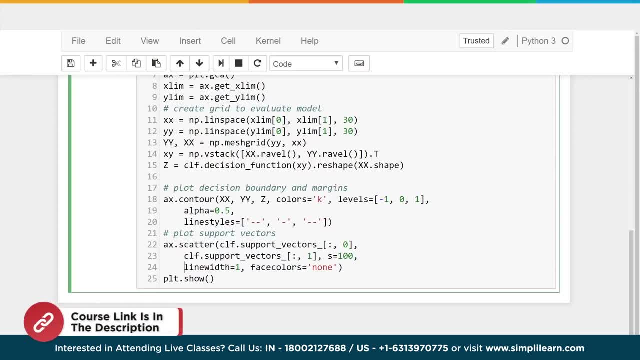 And you'll see that we have the x- x dot shape in here. This literally takes the x- x, resets it up connected to the y And the z value. lets us know whether it is the left-hand side. It's going to generate three different values. 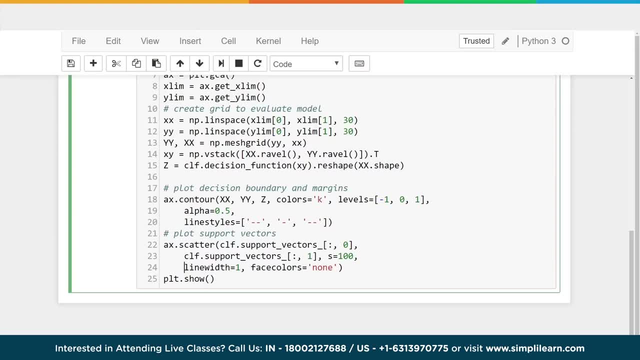 the z value does, And it'll tell us whether that data is a support vector to the left, the hyperplane in the middle or the support vector to the right. So it generates three different values for each of those points, And those points have been reshaped. 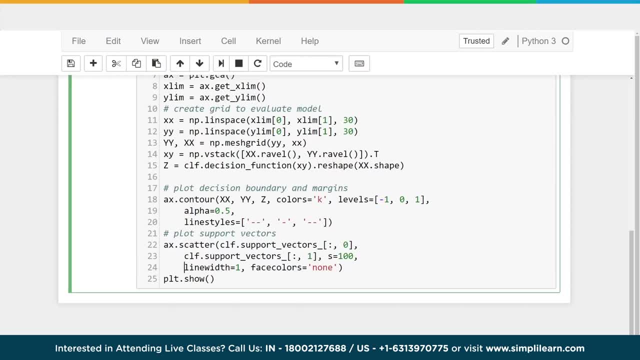 so that they're right on the line, on those three different lines. So we've set all of our data up, We've labeled it to three different areas And we've reshaped it And we've just taken 30 points in each direction. 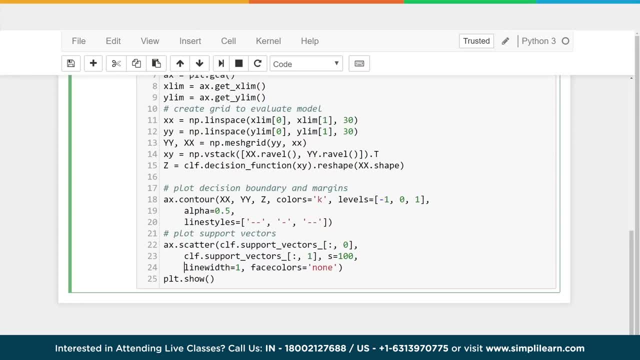 If you do the math, you have 30 times 30, so that's 900 points of data, And we separated it between the three lines and reshaped it to fit those three lines. We can then go back to our map plot library. 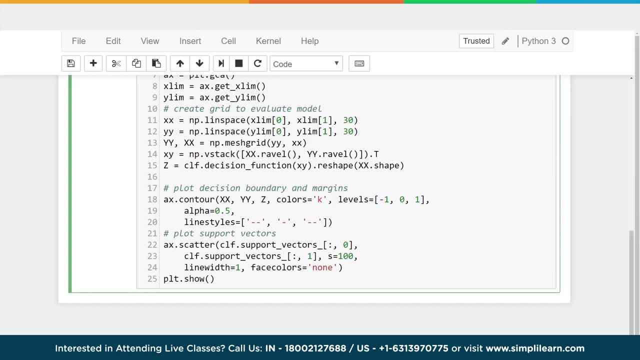 We've created the ax and we're going to contour And you'll see, here we have contour, capital XX, capital YY. These have been reshaped to fit those lines. Z is the labels. So now we have the three different points. 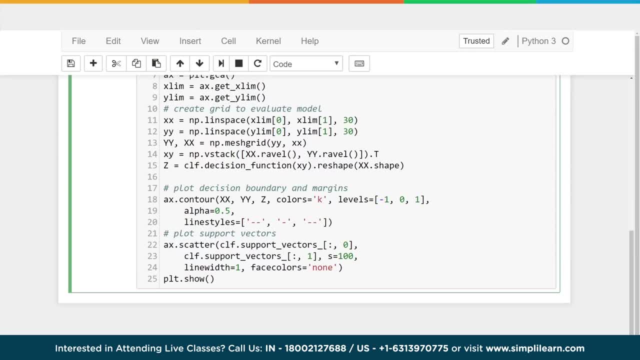 with the labels in there And we can set the colors. equals k And I told you we had three different labels but we have three levels of data. The alpha just makes it kind of see-through, So it's only 0.5 of the value in there. 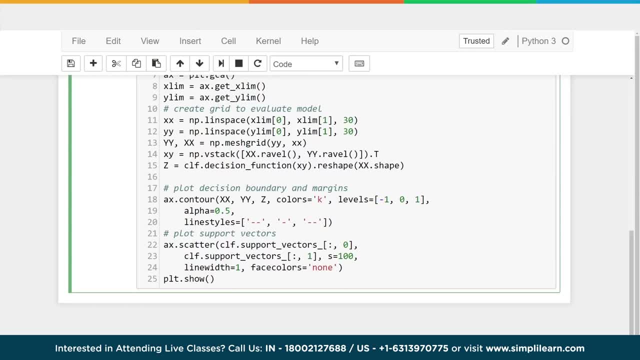 So when we graph it, the data will show up from behind it wherever the lines go. And finally, the line styles. This is where we set The two support vectors to be dash, dash lines, and then a single one is just a straight line. 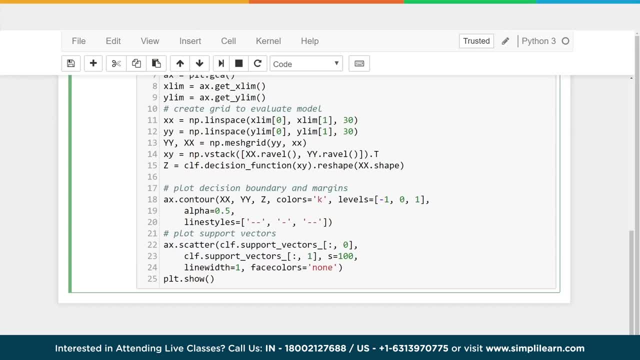 That's what all of that setup does. And then, finally, we take our axscatter. We're going to go ahead and plot the support vectors, But we've programmed it in there so that they look nice like the dash, dash line and the dash line on that grid. 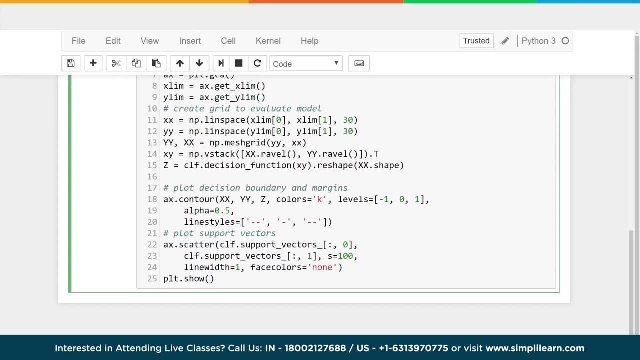 And you can see here, when we do the clfsupport vectors, we are looking at column 0 and column 1.. And then again we have the s equals 100.. So we're going to make them larger And the line width equals 1.. 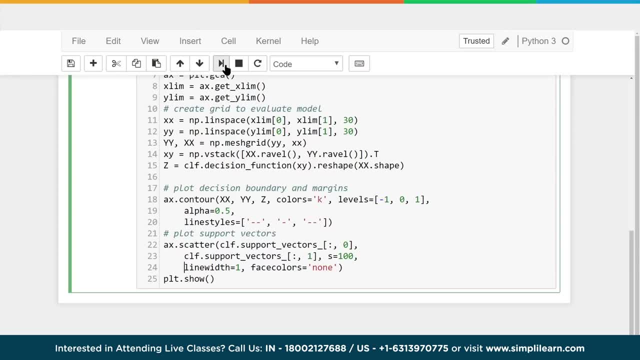 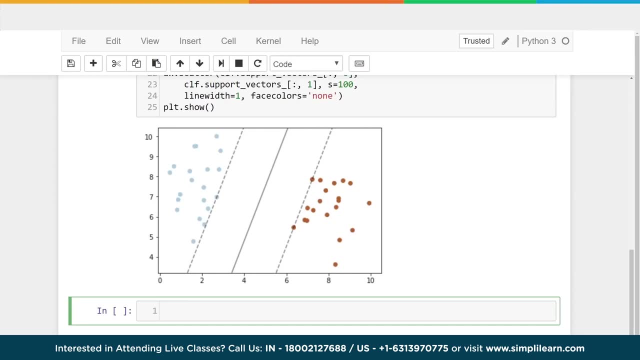 Face colors equals none. Let's take a look and see what that looks like when we show it And you can see when we get down to our end result. it creates a really nice graph. We have our two support vectors and dash lines. 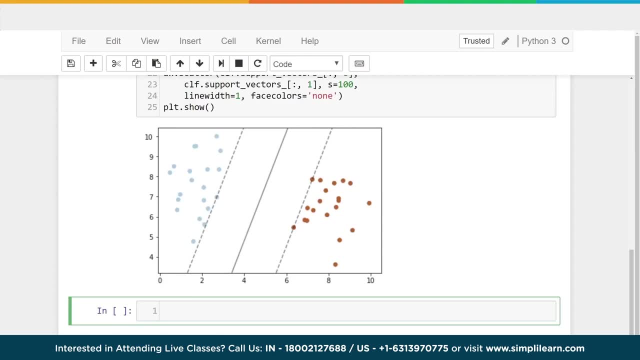 And they have the near data. So you can see those two points, or in this case the four points where those lines nicely cleave the data, And then you have your hyperplane down the middle, which is as far from the two different points as possible. 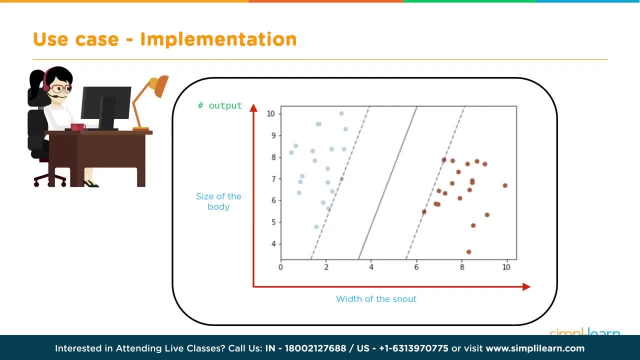 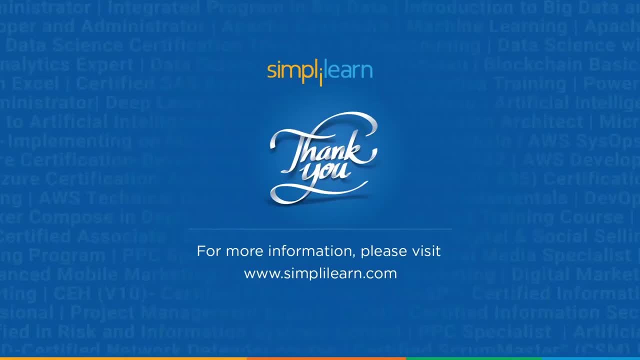 creating the maximum distance. So you can see that we have our nice output For the size of the body and the width of the snout, And we've easily separated the two groups of crocodile and alligator. We have reached the end of this session. 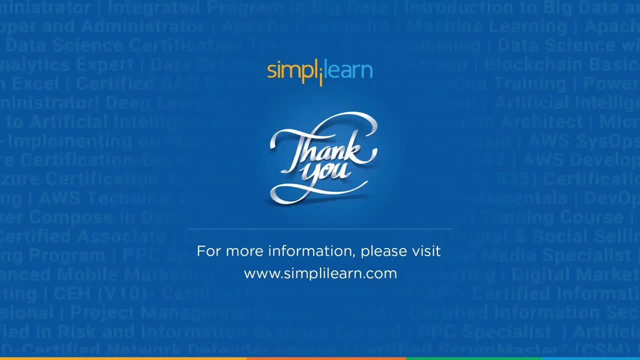 And should you need any assistance, PPT and other resources used in this session, please let us know in the comment section below And a team of experts will be happy to help you as soon as possible. Until next time, thank you, and keep learning.